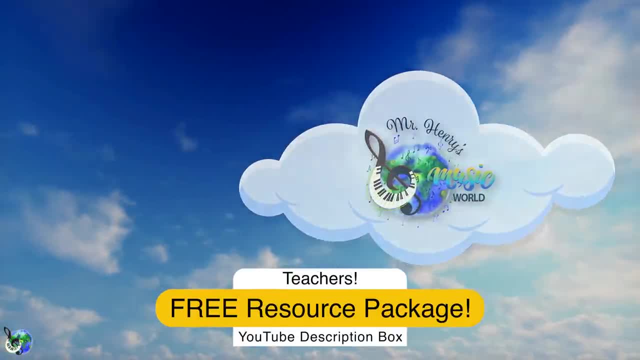 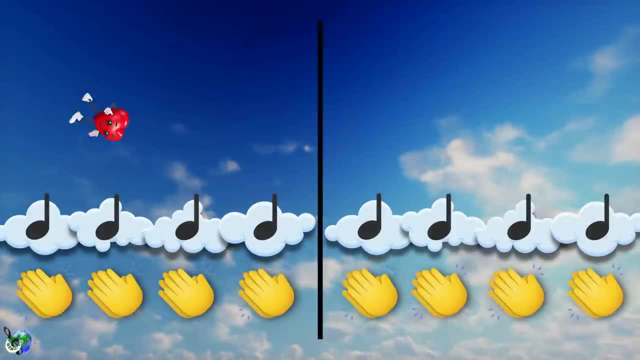 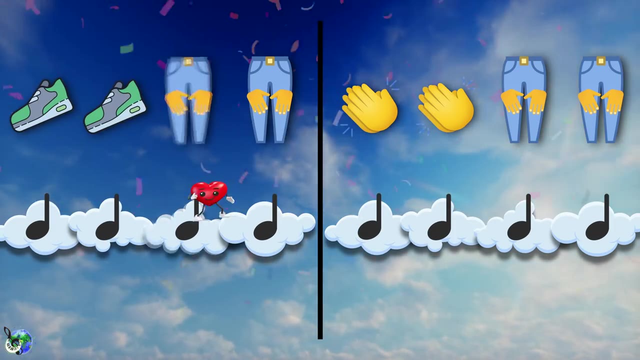 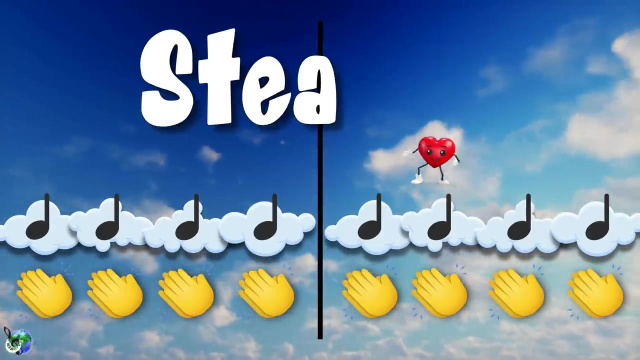 Let's all keep the steady beat. Yeah, stomp, stomp, pat, pat, clap, clap, pat pat. Let's all keep the steady beat. Yeah, stomp, stomp, pat, pat, clap, clap, pat pat. 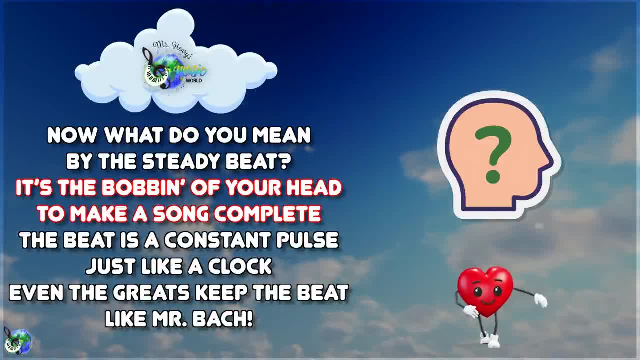 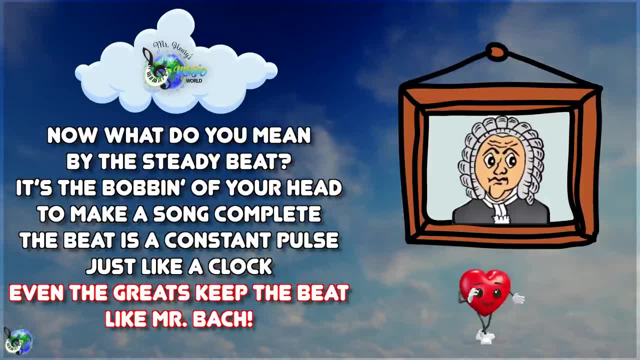 Now, what do you mean by the steady beat? It's the boppin' of your head to make a song complete. The beat is a constant pulse, just like a clock. Even the greats keep the beat. like Mr Bach, Your heart keeps the steady beat all day and night, Thumping fast and slow. now you gotta recite. 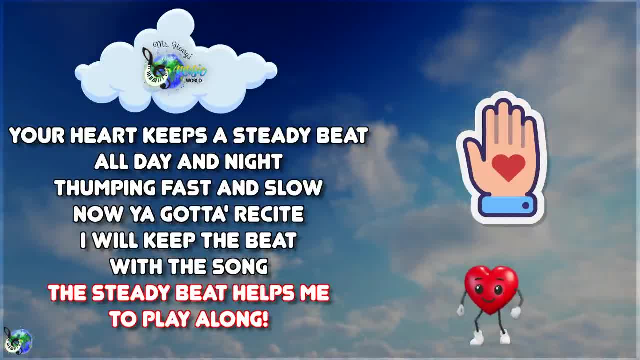 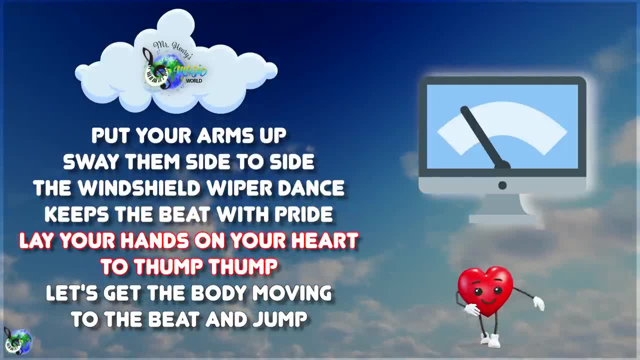 I will keep the beat with this song. The steady beat helps me to play along. Put your arms up, sway them side to side. The windshield wiper dance keeps the beat with pride. Lay your hands on your heart to thump, thump. Let's get the body movin' to the beat and jump. 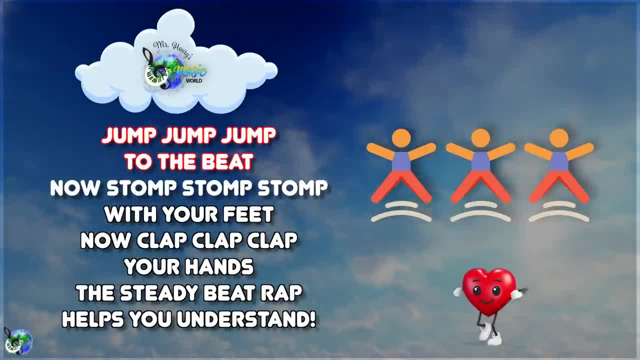 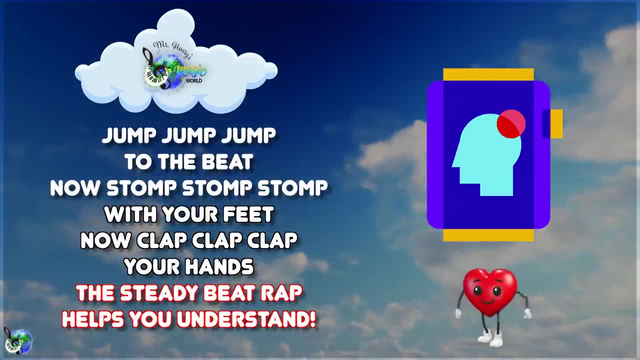 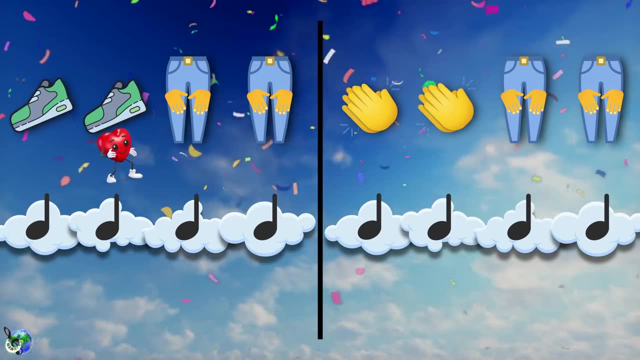 Jump, jump, jump to the beat. Now stomp, stomp, stomp with your feet. Now clap, clap, clap your hands. The steady beat rap helps you understand. Let's all keep the steady beat. Yeah, stomp, stomp, pat, pat, clap, clap, pat pat. 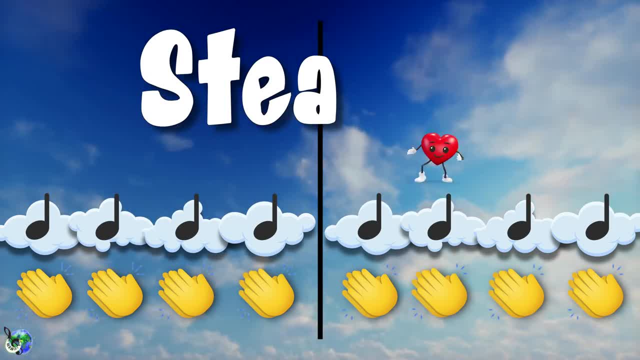 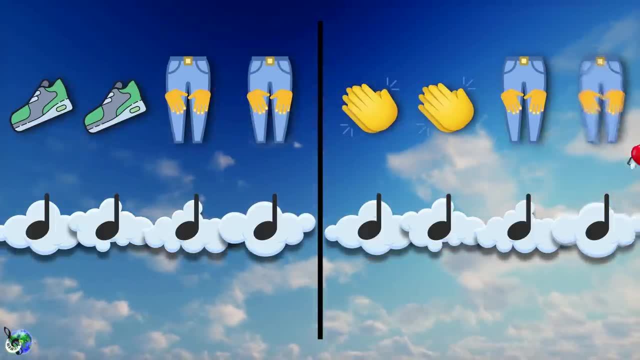 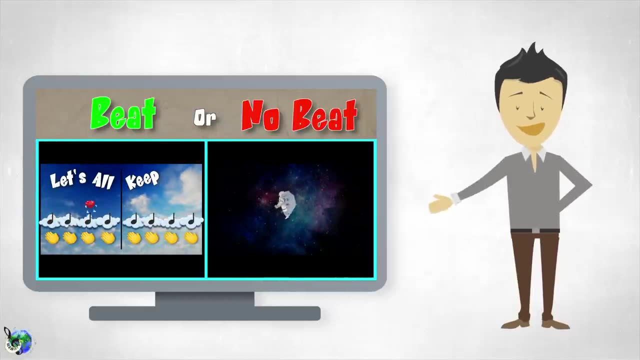 Let's all keep the steady beat. Yeah, stomp, stomp, pat, pat, clap, clap, pat, pat. Alright, Are you ready to keep the steady beat in your feet? Let's play a game to figure out if the music has a steady beat or no beats at all. 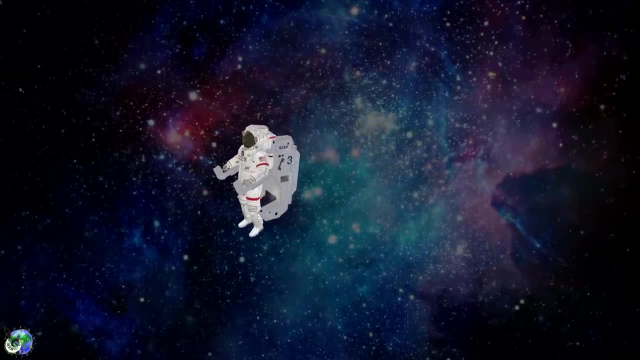 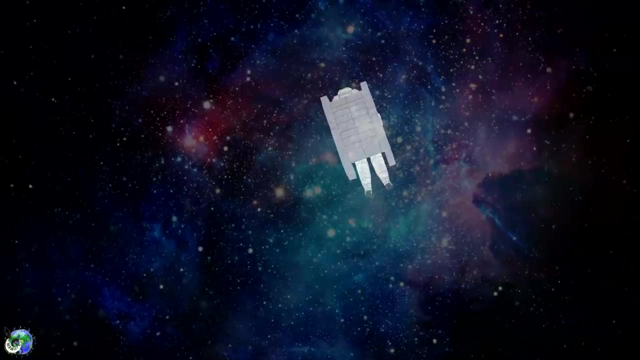 Way to tickle. No beat at all. That's right. sometimes music has no beat. Take a listen. Not having a beat in music is kinda like floating around in space. So if you hear no beat at all, pretend like you're floating around in space. 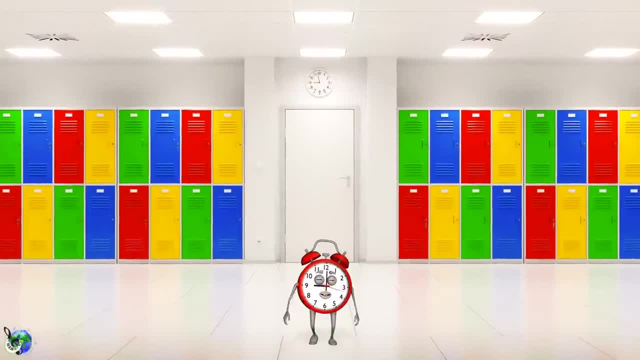 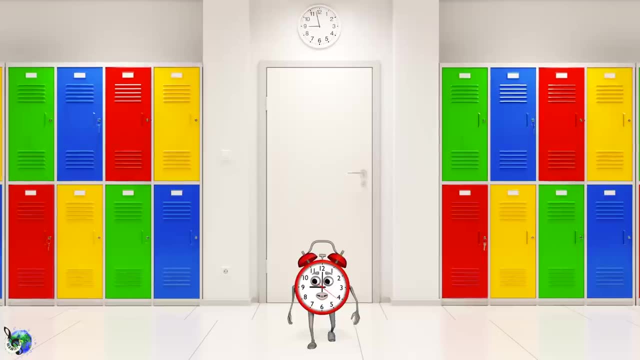 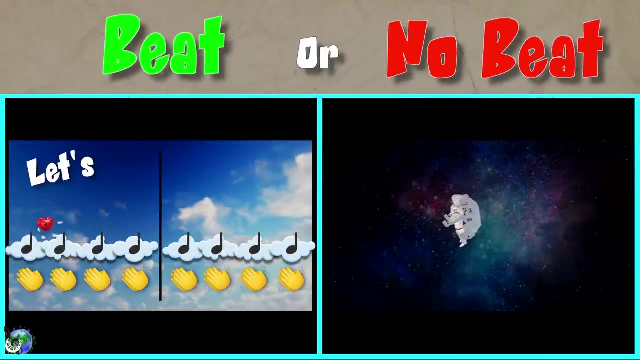 But if you do hear the steady beat, safely march around the room just as if you were in a marching band. Are you ready? Let's stand up, move and figure out. if the music has a steady beat, Go, kicks off. Now, if you have a beat, be ready to hit theUCK. 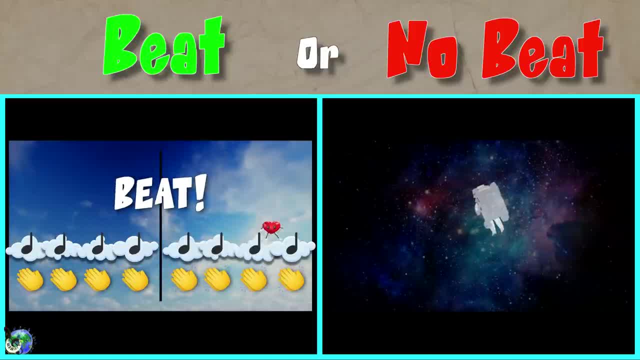 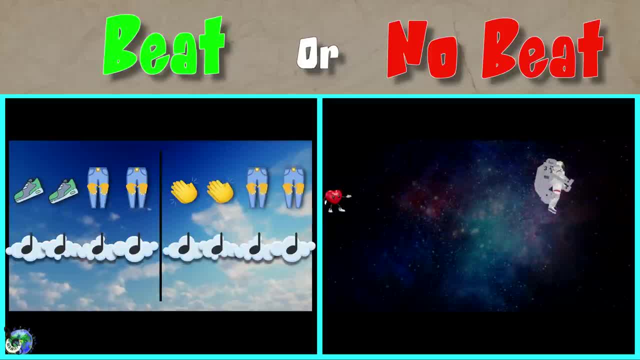 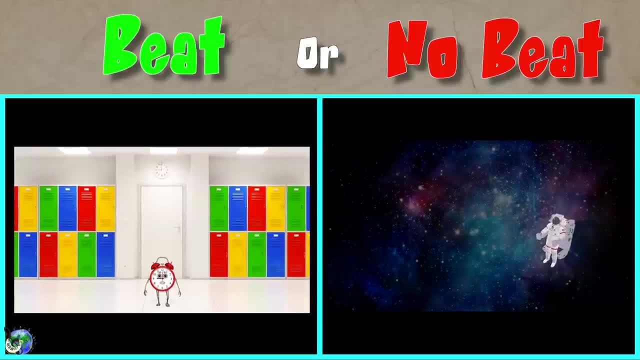 You're ready to get going. If you have a beat and have no beat, Take yourself to the beat. You've got to beat the shit out of yourself. You've gotta make sure you get to the beat, Cause then you're gonna feel like you're on top of the world. 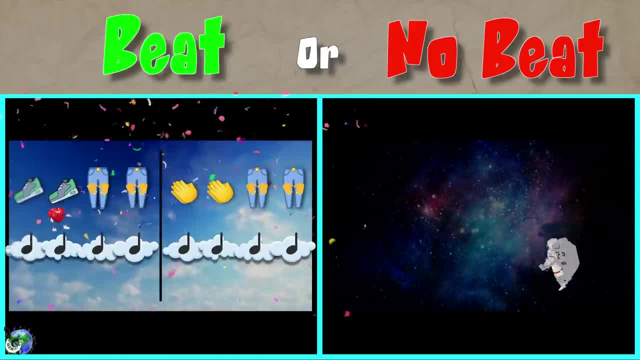 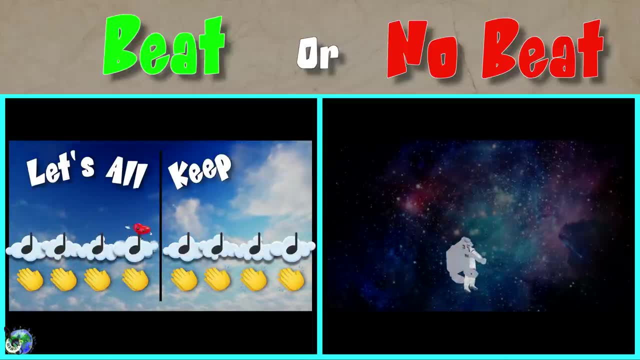 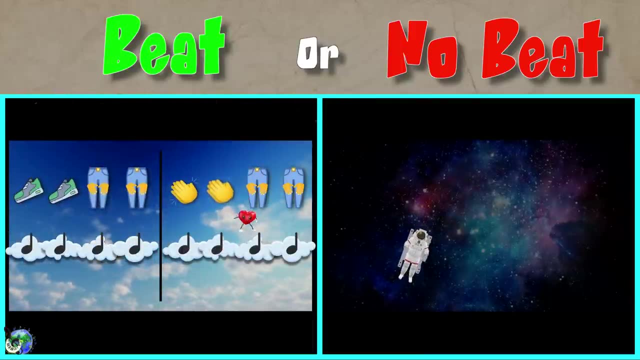 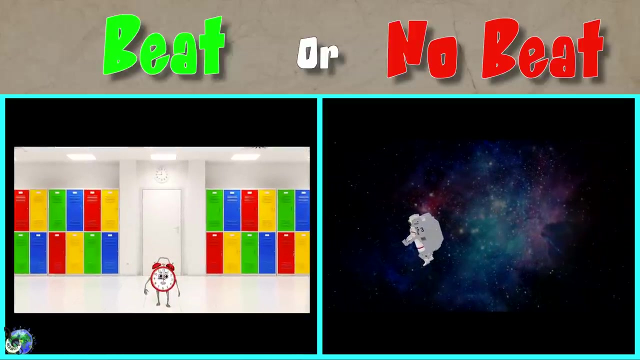 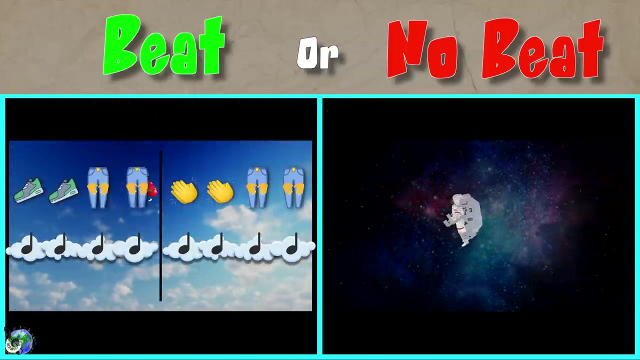 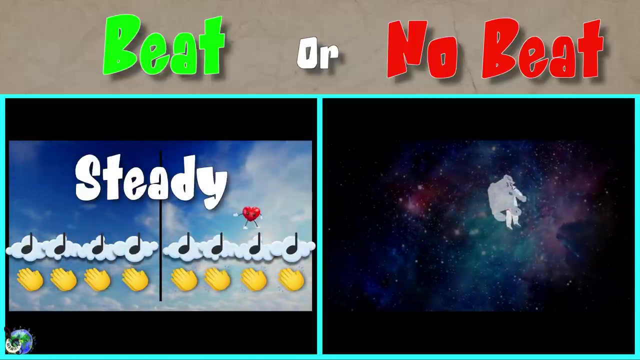 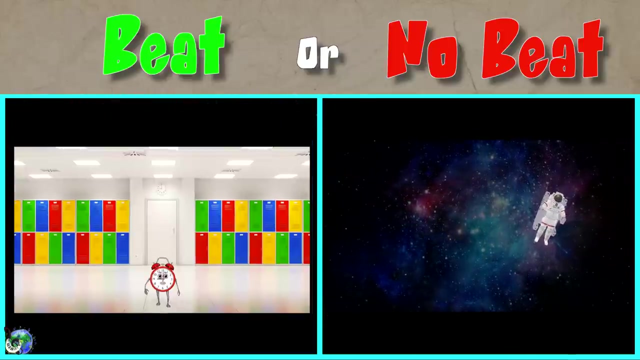 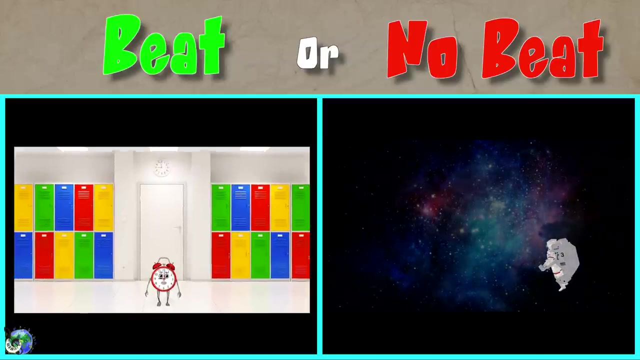 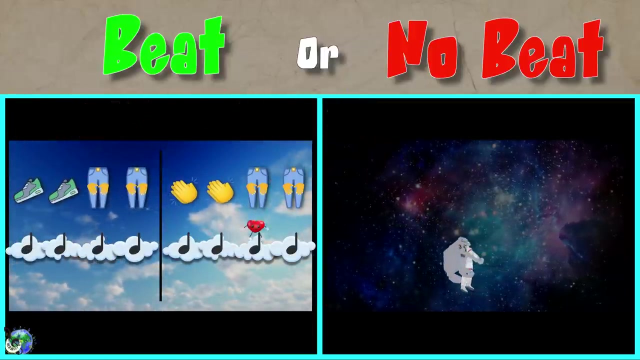 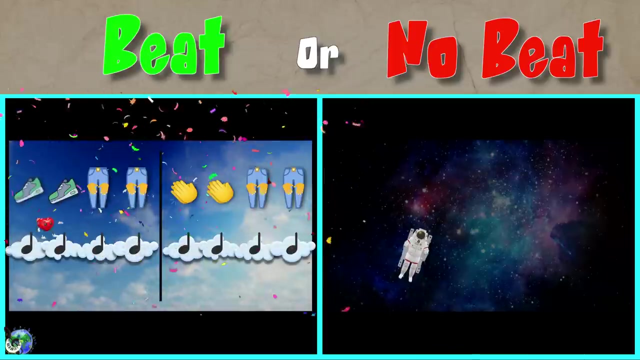 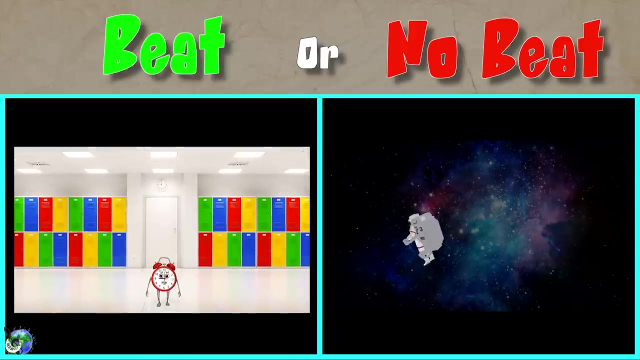 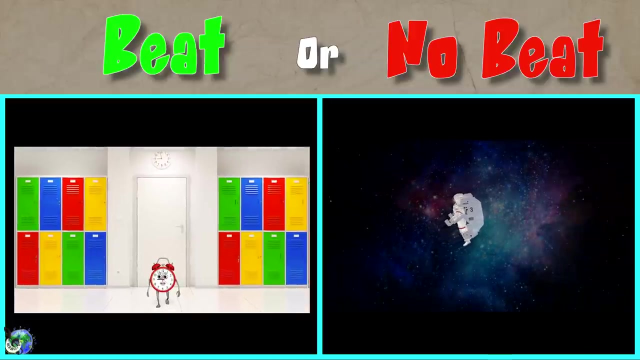 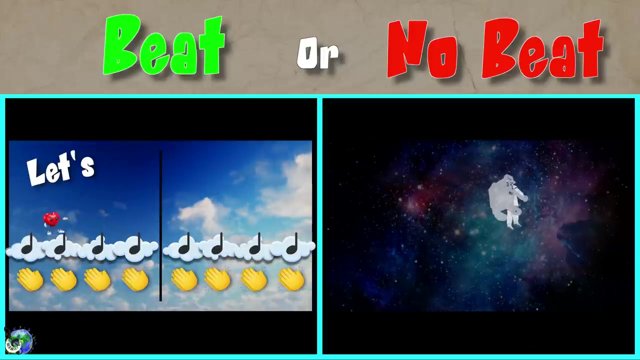 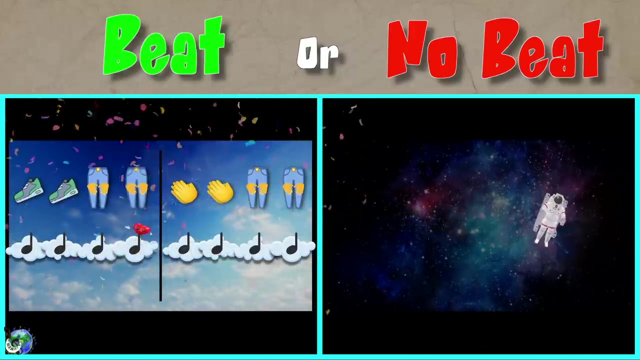 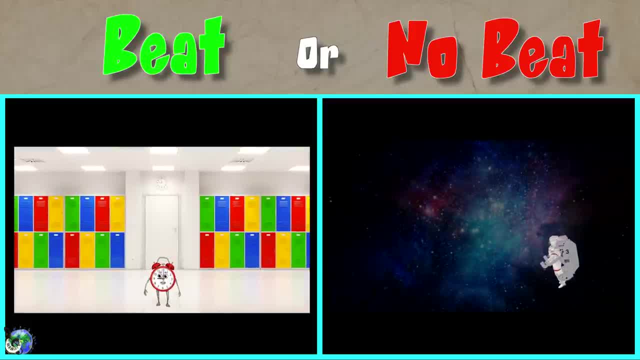 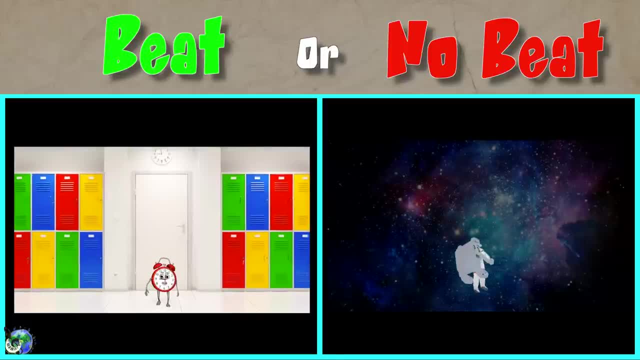 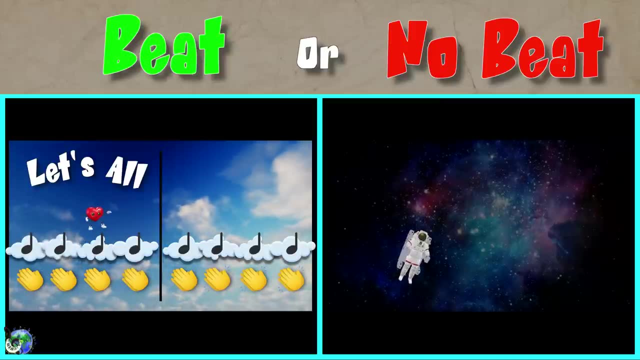 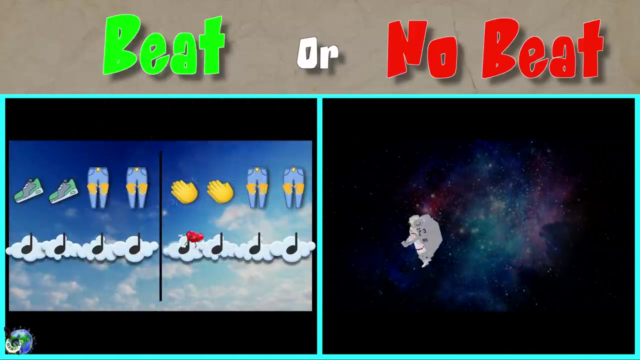 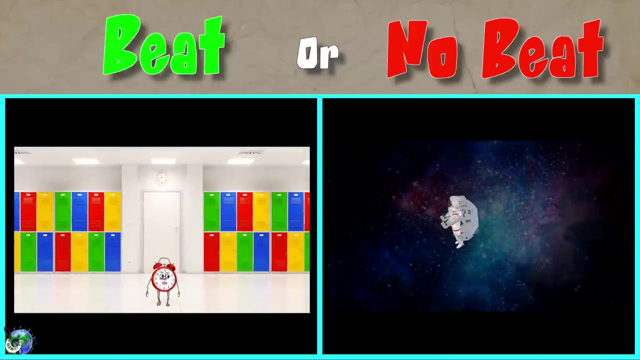 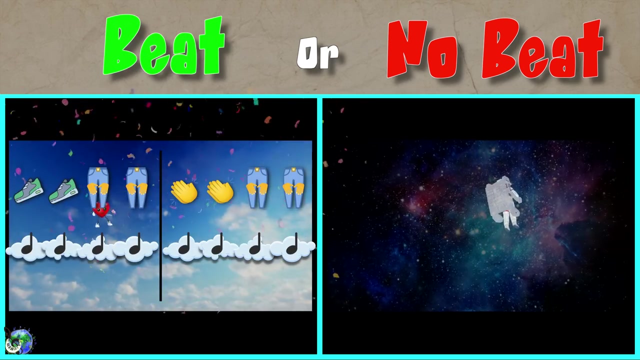 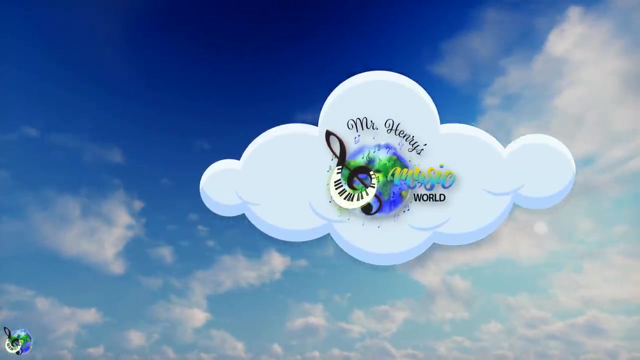 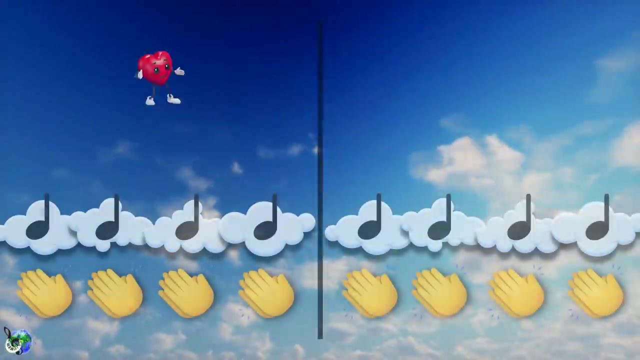 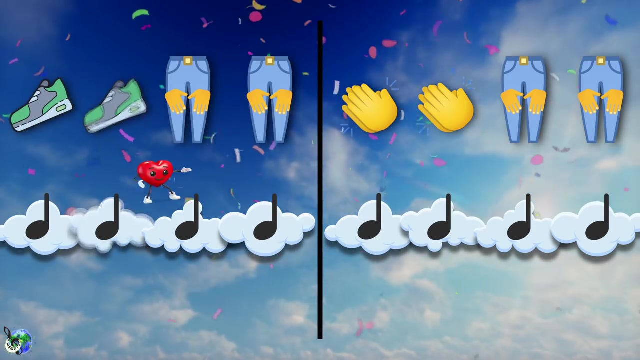 Thank you, Nice job figuring out if the music had a steady beat or no beat at all. Let's get back to singing and performing the steady beat. Let's all keep the steady beat. Yeah, stomp, stomp, Hap, hap, clap, clap.